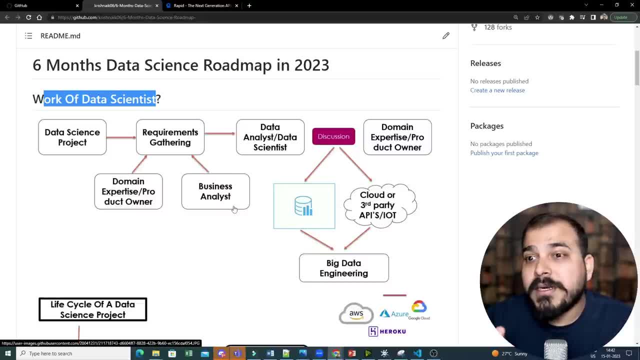 and subtasks and then they will go ahead and create a data science project And then they will provide all these requirements to the data analyst and data scientist team which is in this step two, then this: with the domain expert and product owner will have a discussion to identify the data set. 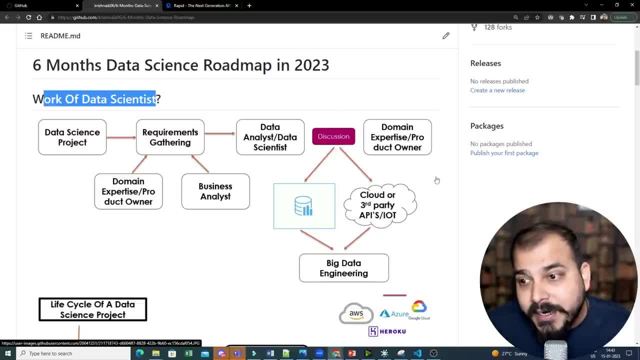 to solve this particular problem. They may be dependent on the internal database or they may be dependent on the third party cloud API. right Now, when I say third party cloud API, many people have actually asked me: what is this third party cloud API? private, like it will also be paid. 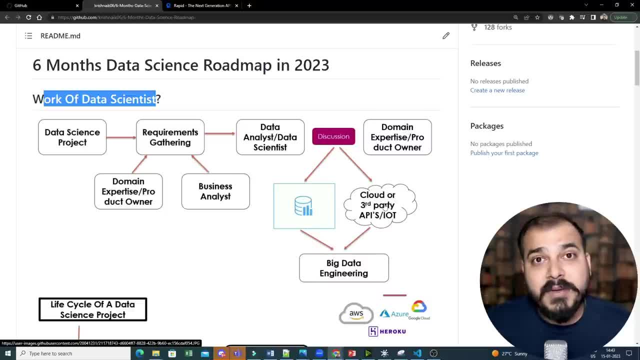 So what are this specific data? Yeah, there are multiple ways, guys. you can also probably create your own IoT team and probably start creating the data set with respect to your products and do it, But there are many business use cases that are common. right In service based companies, you may get projects from different. 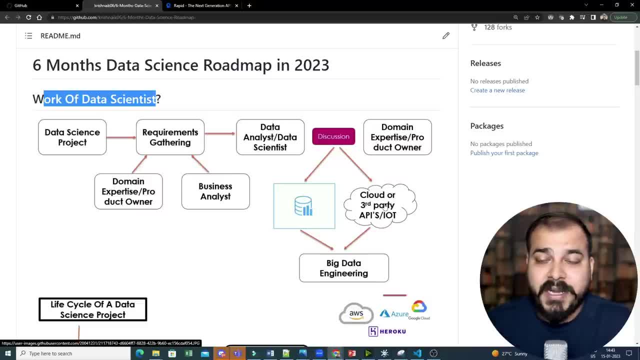 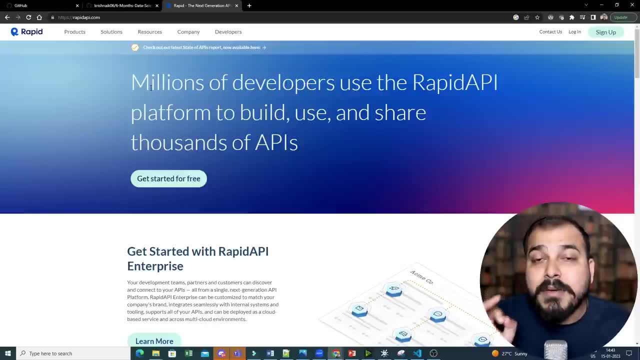 different sectors itself And, based on that, your data may be changing right Now. with respect to that, I have actually checked out this rapid API platform, wherein you will be able to see some amazing public data set. Again, guys, this is not a sponsored video, but I was able. 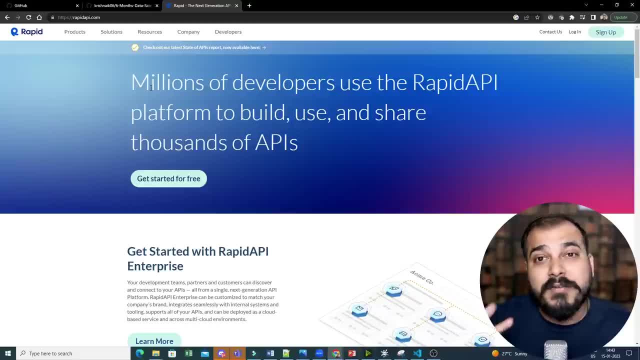 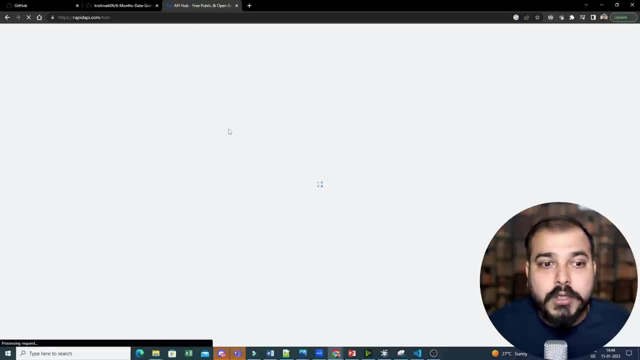 to find it out And this will be super important for you all to solve different, different use cases. So, over here, what you can basically do, just log in over here And, with respect to the login, like Google login, you can actually do And after going over here, you'll be able to see. 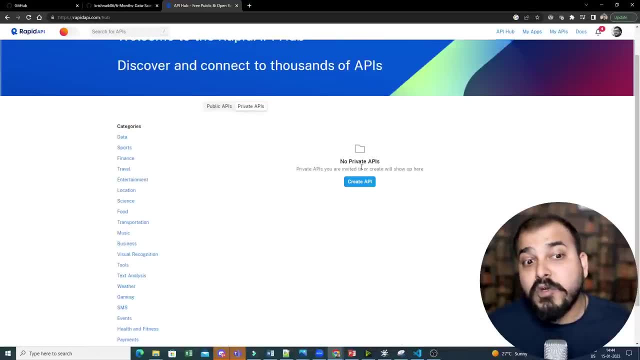 public API's and private API's. Private API's basically means you can also create your API and you can probably do it or upload it over here, right, And basically, like you're creating our API, deploying it in a cloud and you can put that specific API over here. 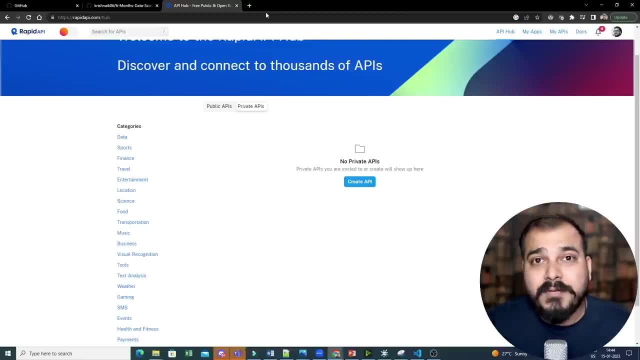 If you want that specific video also, you can let me know. Just in a couple of days I'll also try to upload that particular video. So just write down in the comment how to create your own private API and how to publish in the rapid API. But other than that, 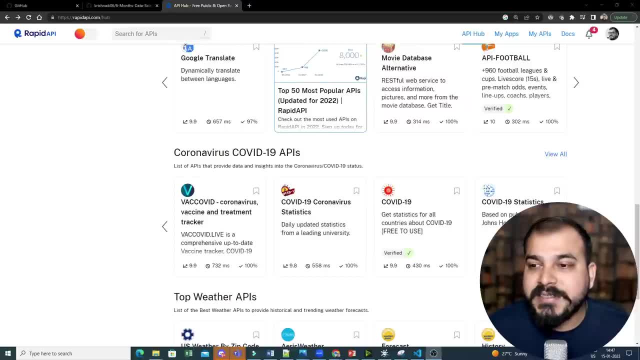 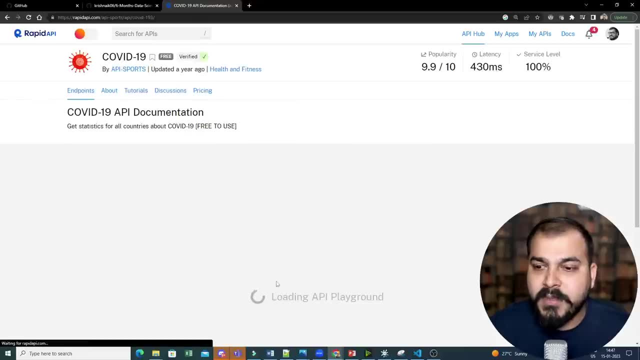 suppose you want to play with public API, you can go over here. So let's say that I want to try any of the specific API's. Let's say, with respect to COVID-19, I'm actually getting this particular API and now this particular API will get loaded here. You will get everything like what all API is. 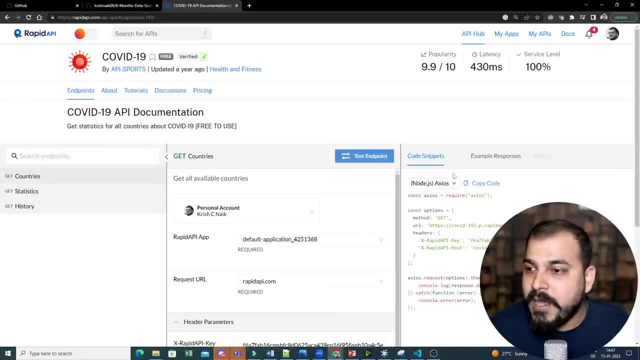 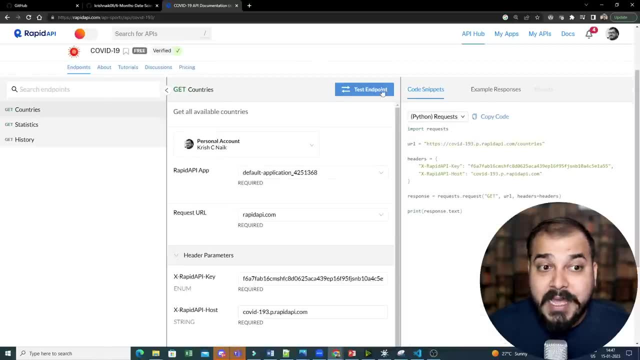 being provided. over here You can have countries, statistics, history, And over here you basically have the code snippet. Suppose, let's say, if I go to Python and probably just select on request- And this is also having all the other programming language- You can probably get the entire code itself. And let's say this: 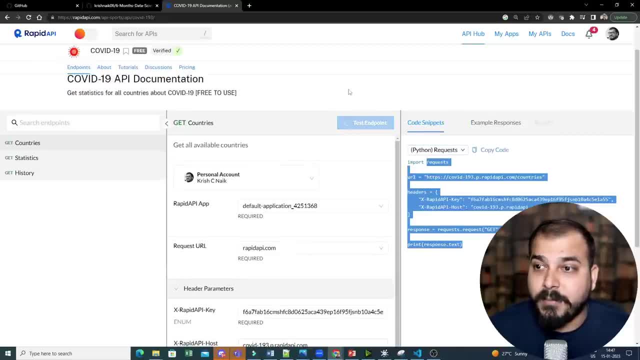 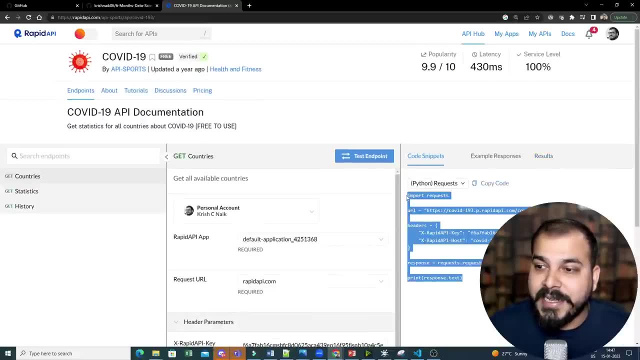 is the code I want to run And here I can also test it with test endpoints. So once I test it you can see that I'm getting all the information right. So suppose if I probably go in the code snippet, I take this up And what I do? I go over here in my VS code, I will just go and execute it. 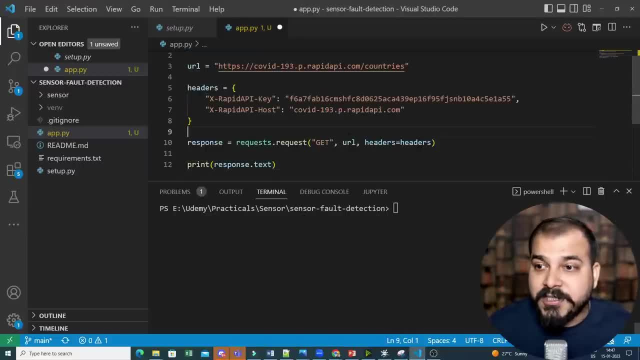 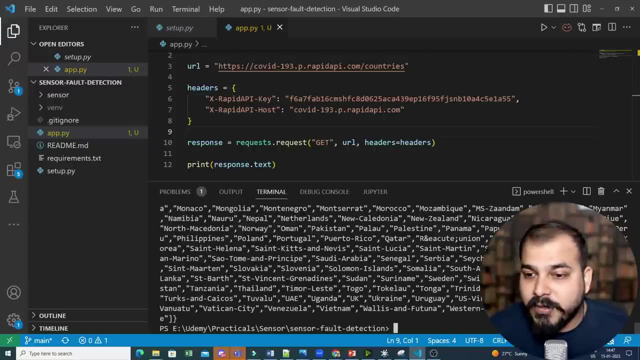 I'm going to clear my screen, Okay, And after clearing my screen I'll just save it over here and I will write Python apppy, right. So here you'll be able to see that I will be also able to get the output. Now, this entire information, I can probably store it in the database or take. 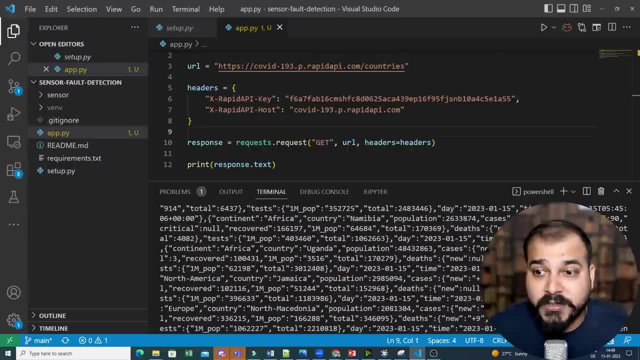 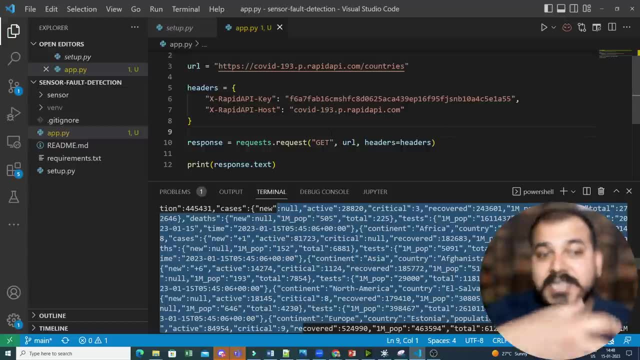 it in any kind of database, like NoSQL SQL database. It is up to you based on the requirement, But here I'm able to get the entire output from that specific API. So my data collection strategies now becomes very simple, right? I don't have to be dependent on. 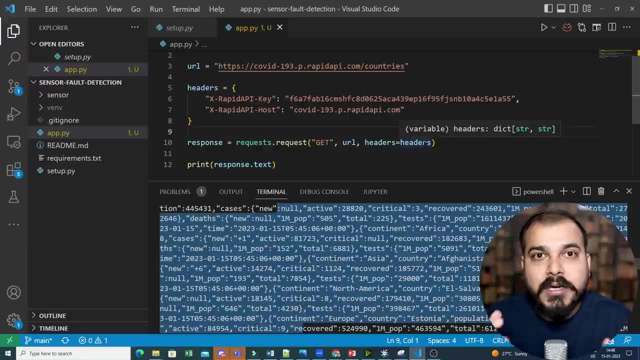 anything else. And this also looks amazing because this is what, in the real world scenario also, we do in industry-ready. when we are solving some industry-ready projects, we have to be dependent on third-party APIs, because these APIs will continuously giving us data with respect to 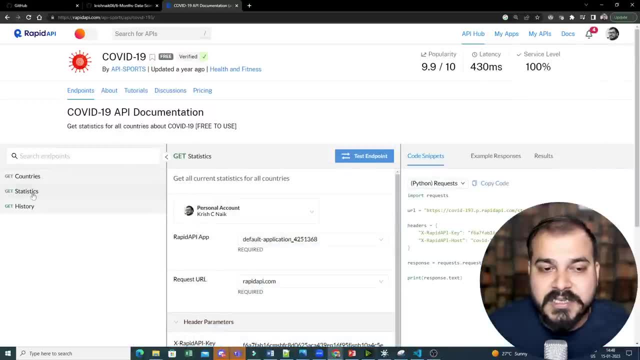 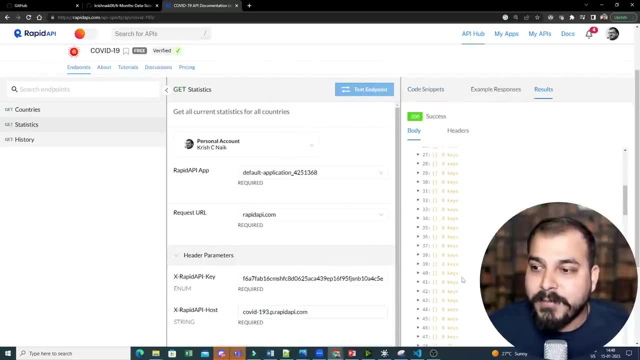 dates right. Not only that. let's say I want to try with statistics. Now, you just see, I clicked on statistics, the entire code changed. I'm just going to copy the code. You can also test the endpoint over here And based on the test, I will be able to get all the answers. You can see that. 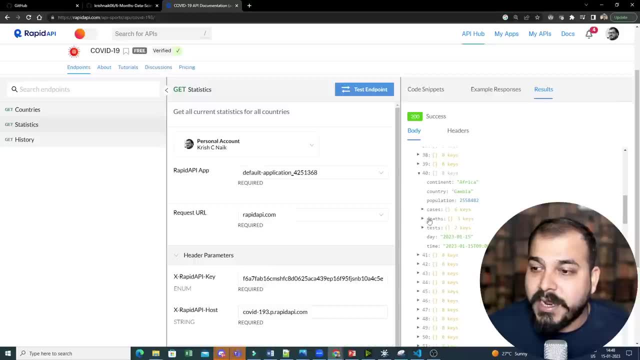 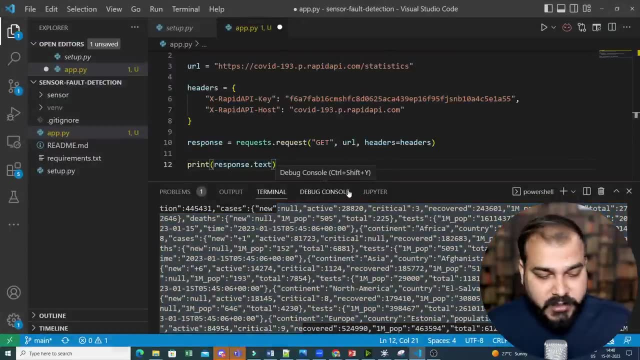 I'm getting with respect to every country and countries. How many cases were there? How many deaths were there? How many tests are there? Everything right. So I will just go ahead and execute it over here. Same code, I'll paste it over here. 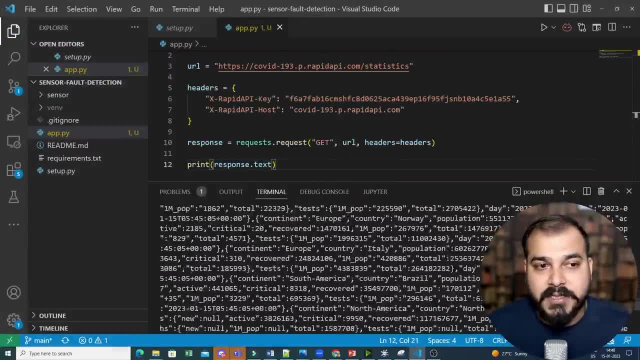 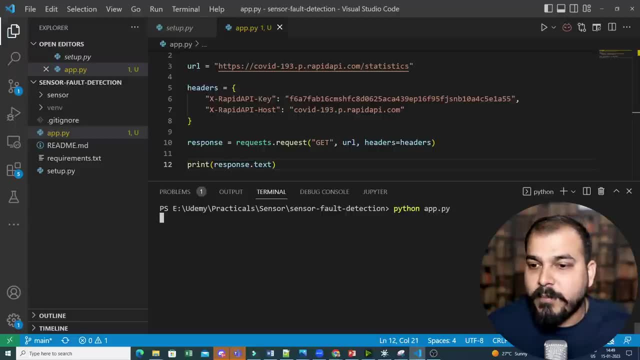 save it And then I will just go and clear the screen. Now see this, how easily I'm able to use this entire rapid API, right? So I'm just going to write pythonapppy And finally you'll be able to see I'm getting all the output. Now, what I can do, I can probably take this output. do some. 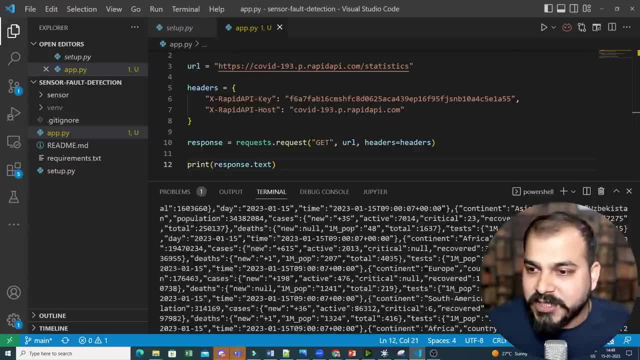 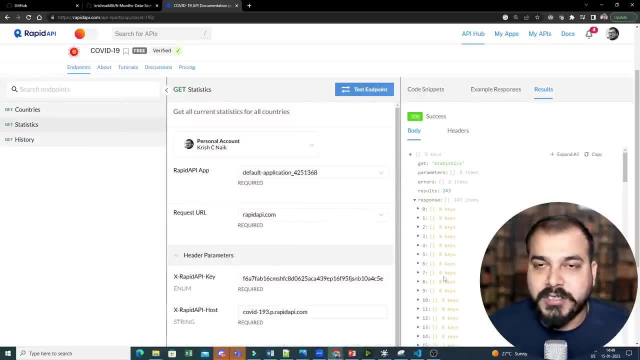 pre-processing and store it in the MongoDB- right? It is obviously in the JSON format. If you directly go to MongoDB, you will be able to get the output like this: only right With respect to all the records, right. This is how you can basically try it out Again. guys, here you also have paid API. 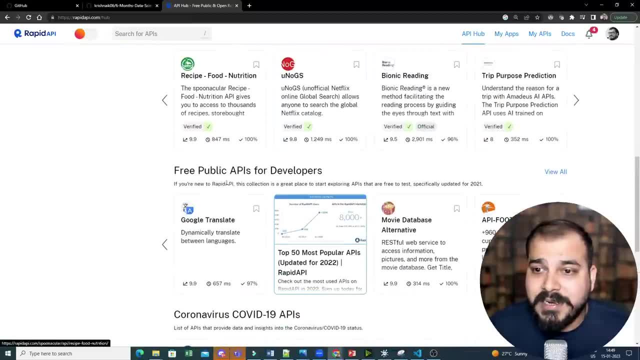 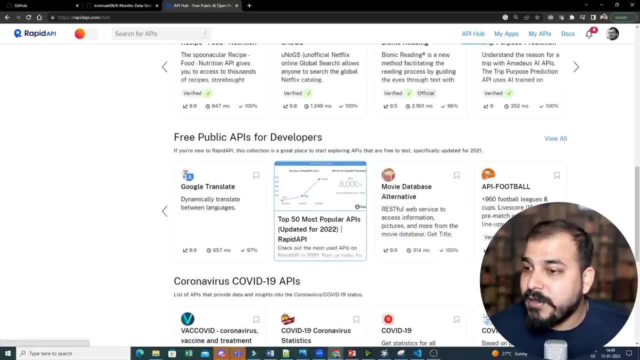 So suppose, if I probably go to rapid API, I want something else, Let's say free public API for developers. So here I have top 50 most popular APIs. right, You have API football movie database. Now see, many of you implement movie recommendation system. Why can't you directly use the movie? 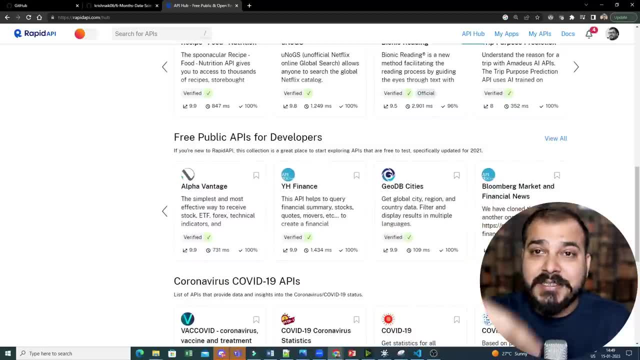 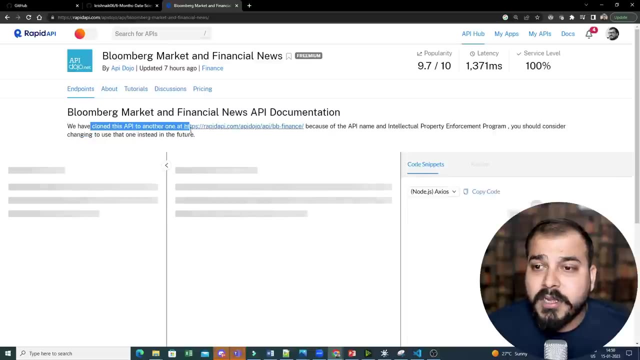 database from here And from there. the data collection strategy is more about reading from some APIs, storing it in the data databases, doing some pre-processing and all See. now here you have Bloomberg, market and financial news API documentation. Let's try this also. We have cloned this API to another. 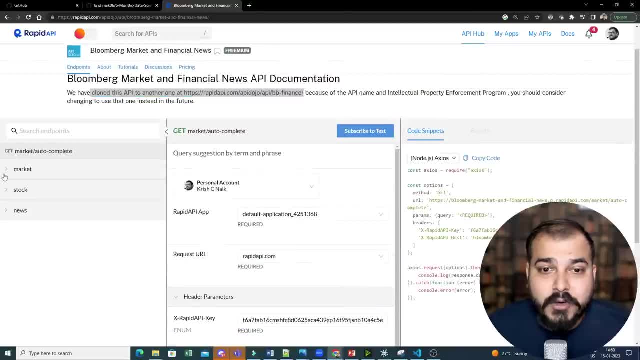 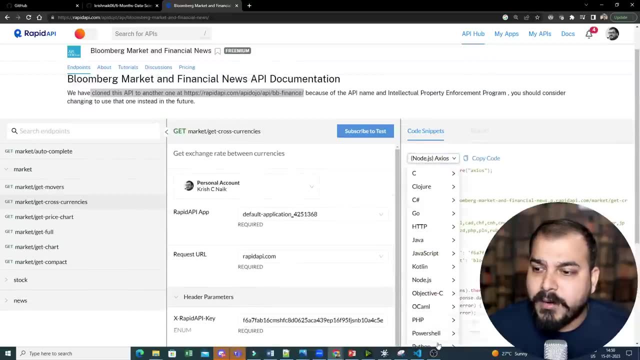 at this API itself. Now, here you can see, here you have market information, get movers, get cross currencies. Let's say, I want to get cross currencies, okay, And I will probably go and just go ahead and get the Python code. So this is my Python code. you can see From this particular 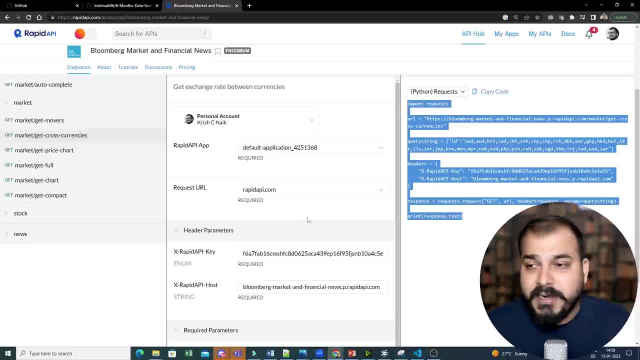 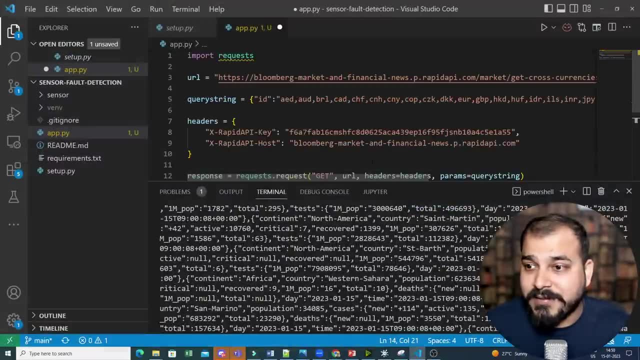 URL we are able to get by using this rapid API key right, And the best thing is that you can also create your own And you can also get paid from this right, Because there are some requests with respect to that. Let me just check one more thing Over here. I have to. 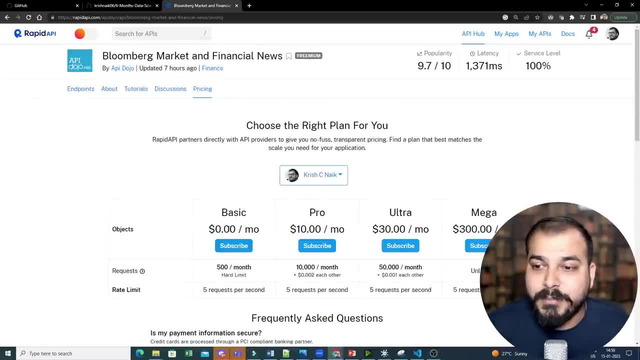 subscribe to this particular test. So once I subscribe it, here you can see B6. Pro Ultra Mega is there. if you probably create your own API, you can also sell it id. Okay, so I have create my own API. you can also sell it ided. okay, I have to subscribe to this particular test, so once I subscribe it, 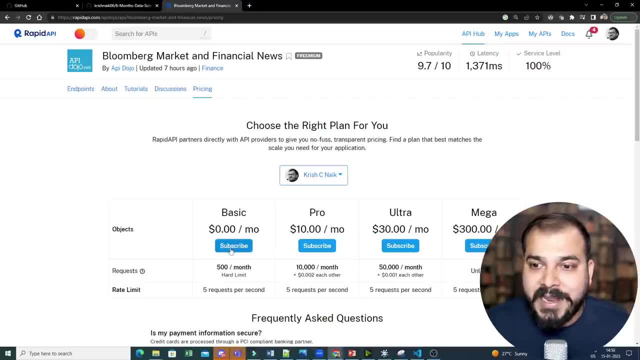 subscribe it. here you can see basics pro ultra mega is there. If you probably create your own API, you can also sell it. OThat will give you the material. you've generated own api. you can also select it. okay, and with the help of chat, gpt, i think it will become very easy. 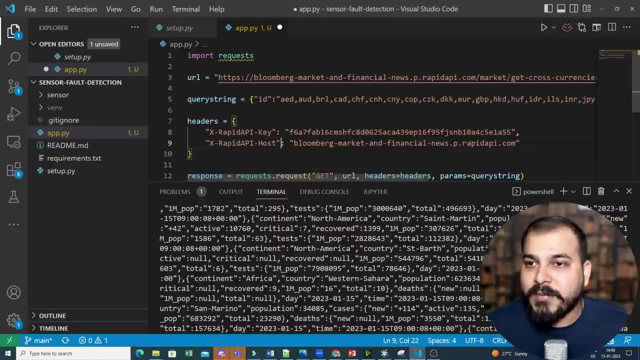 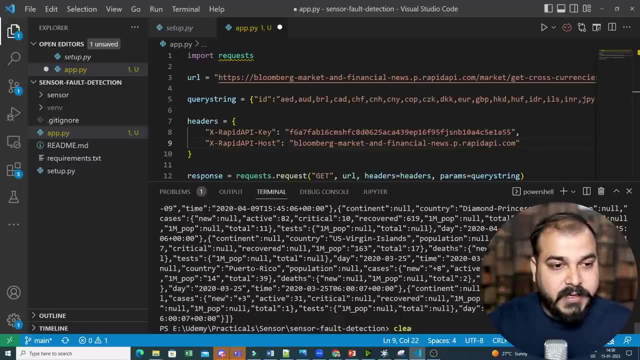 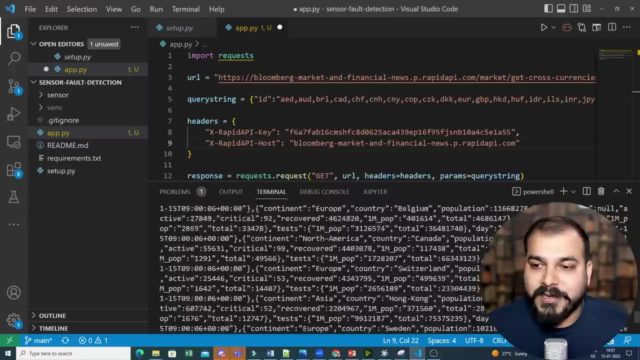 so i'm subscribing to the free one. now i have the code, i'm executing it over here. now let's see whether i'll get the output or not. okay, so i'll just go over here, i will clear the screen and here is my python apppy. so finally you'll be able to see i'm getting all the output, right. 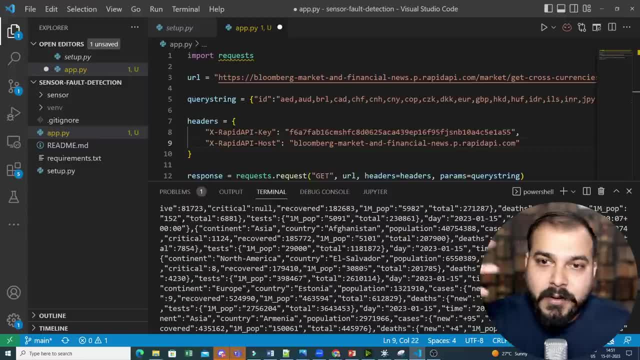 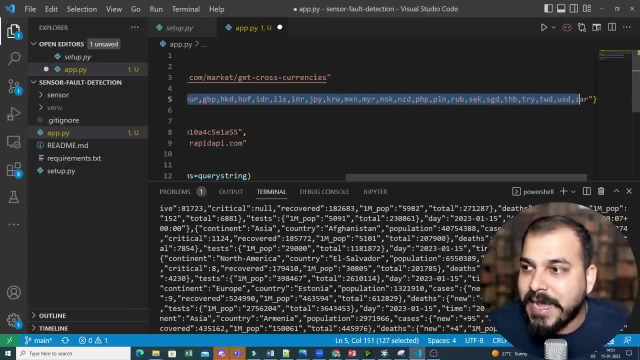 isn't it very easy? you just need to do one or two rounds of processing to get the data in the right format and probably directly use it. so with respect to this query string- all these currencies- i'm able to get all the information right, so i hope you are able to understand, guys, now if i go. 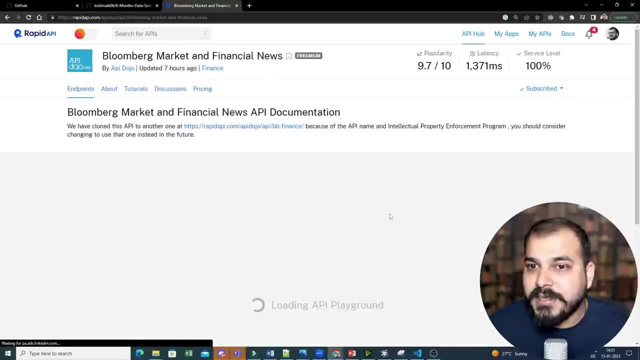 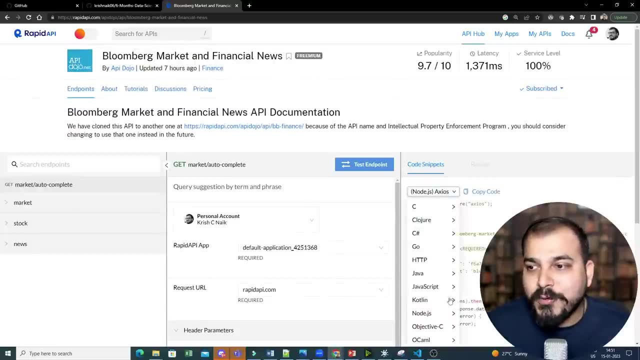 to back to all the plans and probably, if i go to endpoints here, you will be able to also test it out entirely. so any apis over here will be there. just let me know, whether you want to know that, how you can probably earn money from this, because you can also create your own api and probably 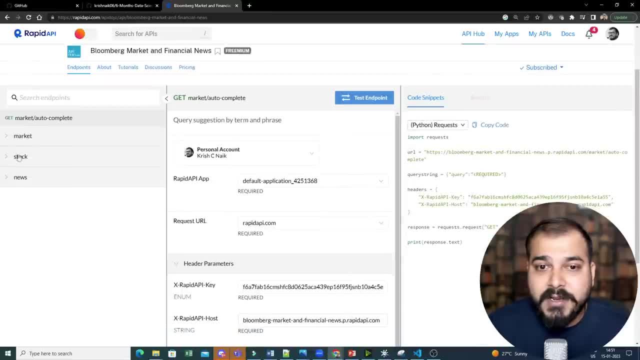 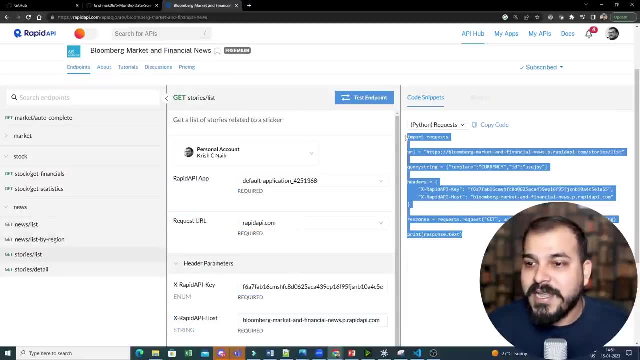 deploy it in some server. you can also create your own api and probably deploy it in some server and probably deploy it in some server and put it over here, right? not only this, i have news news, news list, news list by region, stories list, so if i probably also execute this, i will also be able to get the information, suppose. 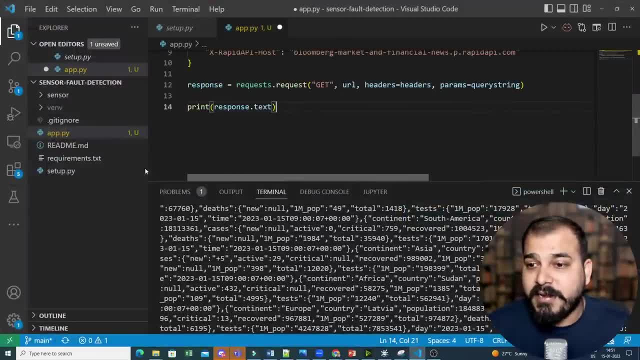 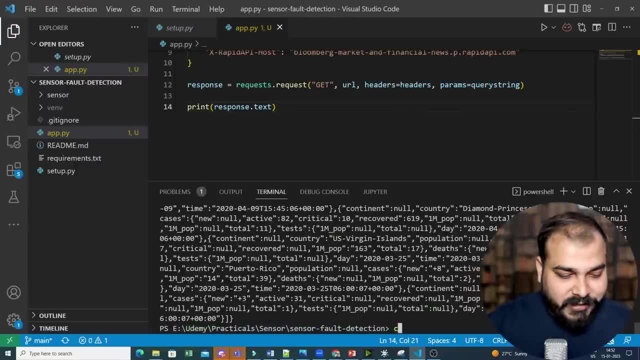 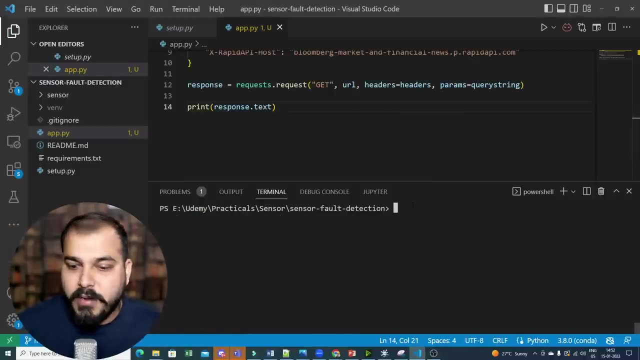 if i'm solving any use case, i'm able to solve most of the things right. so here it is very simple, very easy, and this actually looks like a real world industry project, right? so i'm just going to clear it. let me just make my face go over here, right, and here you have. 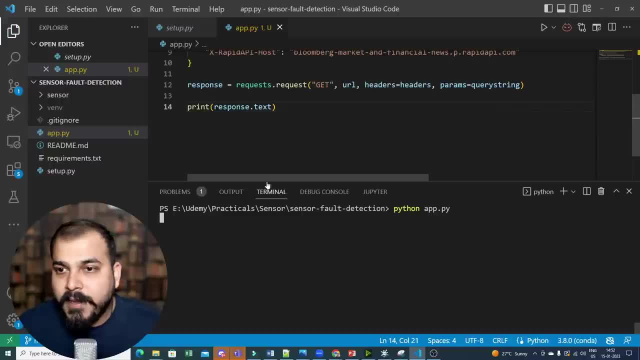 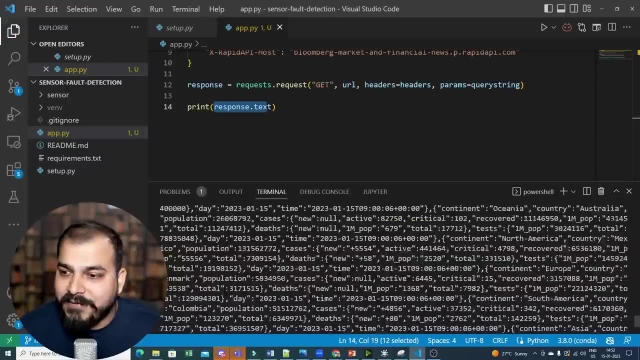 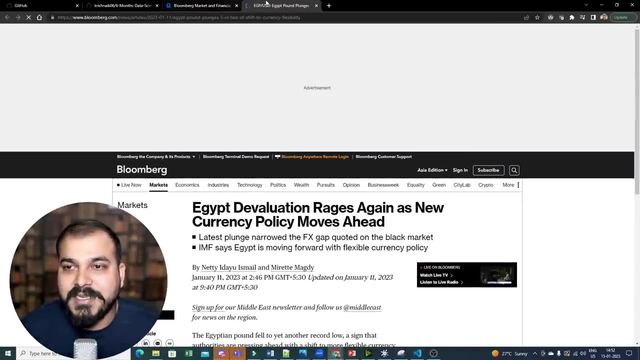 python app dot p1 right and i'll get the response dot text and probably i can also get it in the json format or however. i want see all the links. everything is basically over here. this news article is basically coming. i can also open it over here and see all the information everything. 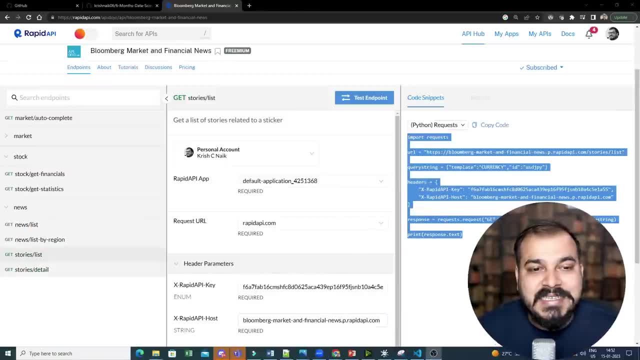 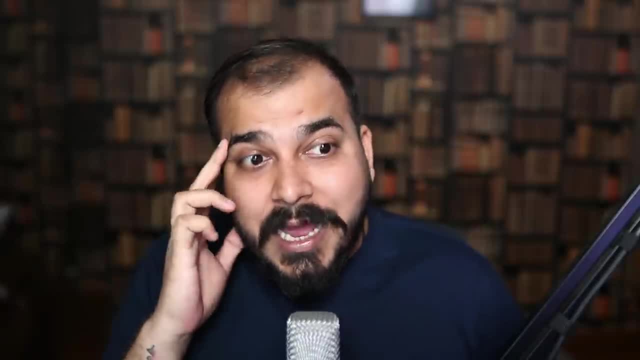 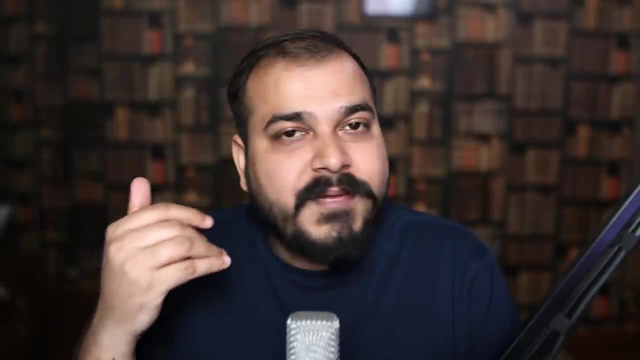 is there right? so this is how you can easily work on the data store data collection strategy itself. you can design it, you can use database. now you're probably thinking like you continue getting the data, you can also create a chrome job every day. uh, probably at some specific time you. 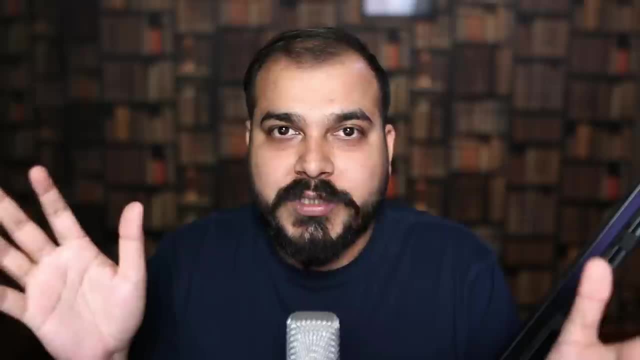 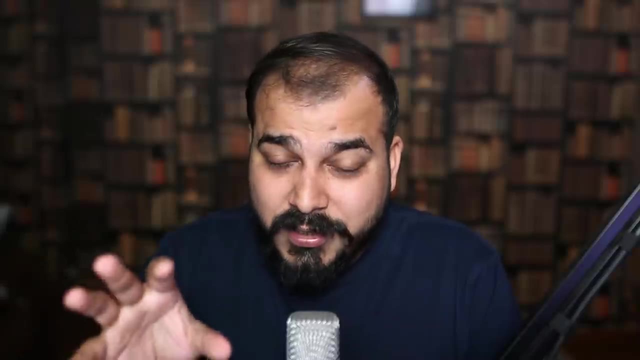 just check the new status and probably upload it in the database and use it right. so this is an amazing way to check it out. rapid api. again, this is not a sponsored video, but yes, i found out this- a good way of actually showcasing your experience, even in companies, if you're probably 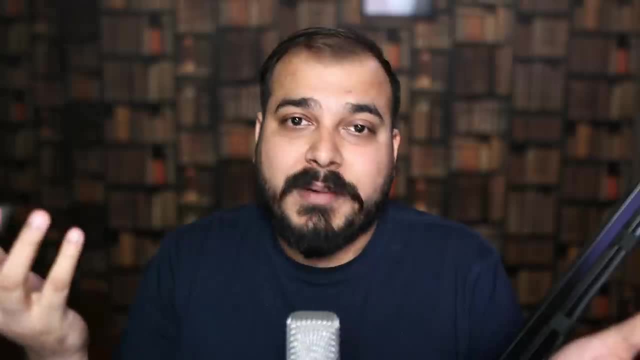 using it. try to use the public api and then try to take the pricing itself, based on the api set, right. so this was it from my side. i'll see you all in the next video. have a great day. thank you, vandal. bye.